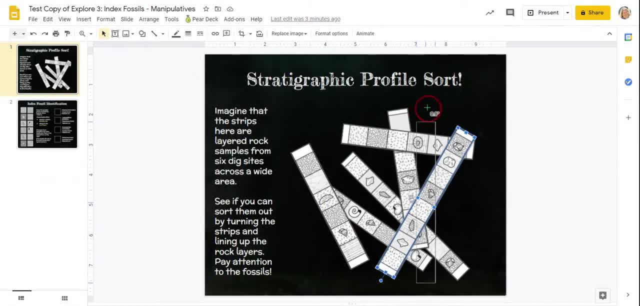 talking to a mouse. You want to swing it up, to turn it upright. Just a hint: the handle should always be at the top. If you try to do it at the bottom, you might mess yourself up. It's also best to do this with these up and down due to the law of superposition, otherwise you won't be able to. 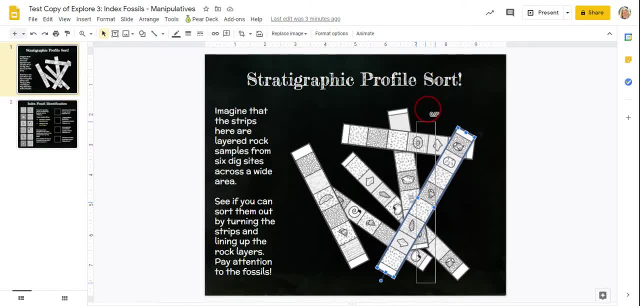 see which layer is oldest and which one is not. Notice that when I have it in this position, I have not let go of the mouse button yet and it says 0.0 degrees. That tells you that it's exactly vertical. Then you can let go and you're good to go. 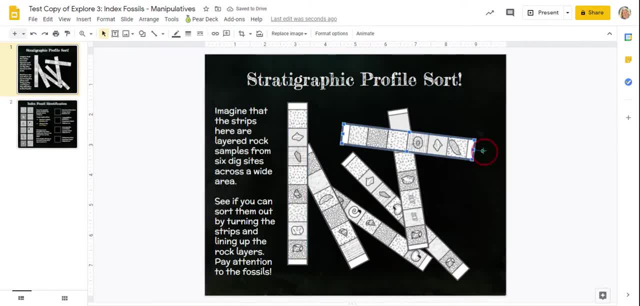 And then you can move it over here. So basically, your first order of business is just going to be to get all these guys straightened out, And holding down shift will make them snap to zero degrees. It'll make them snap vertical much more cleanly, So I recommend doing that as well. 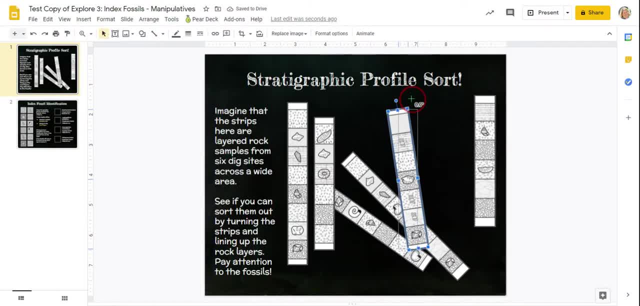 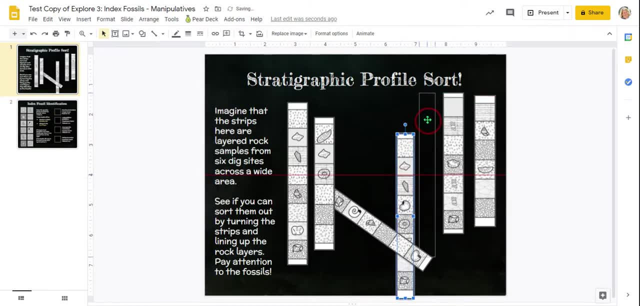 And as you do it, you can just kind of move them out of the way just to get them where they need to be. Okay, And some of these are going to be thicker and some are going to be thicker. And some of these are going to be thicker and some are going to be. 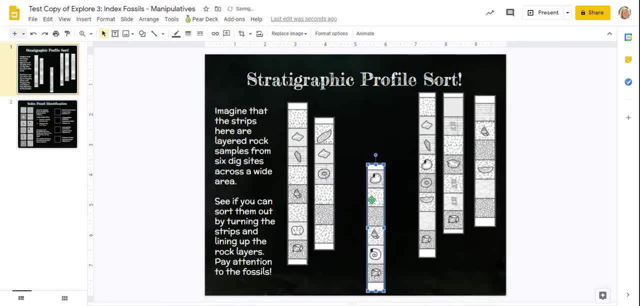 thicker And some of these are going to be thicker and some are going to be thicker, thinner. that's just the nature of dealing with, um, rock layers, i guess. so once you have them all more or less right right side up and you can click on and make sure that that handle there is at the top, 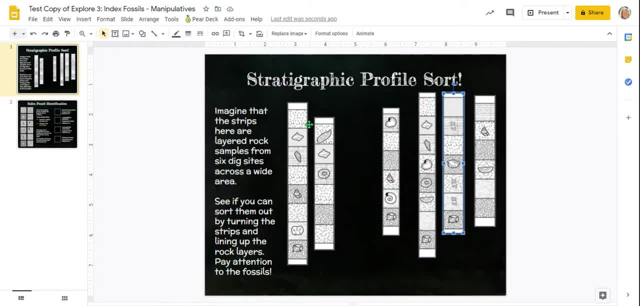 of each one. um, then you gotta line them up. so then what you're looking at is the background, which is where the you know these little flags or stripes or things are, and you want to try to get them so that you're matching all of the layers that are visible on the strip, and it should be possible. 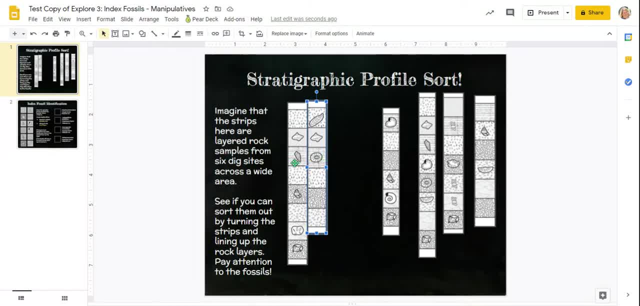 to do that. so you know you want to match the speckles with the speckles, the stripes with the stripes, etc. now they're not going to be 100 clean in how they line up. so you don't have to resize anything. you can just leave it the way it is. but just know that sometimes it's not going to line. 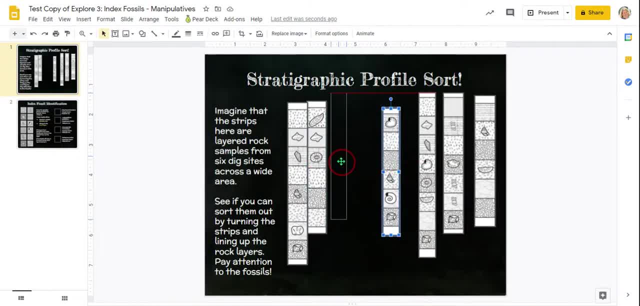 up perfectly, and that's okay. the main thing is just trying to get it as close as possible. so that's, i'm going to move that one down a little bit. see how that lines up there. um, we'll take this one. let's see, right about there, i'm gonna pull this one down just a hair. 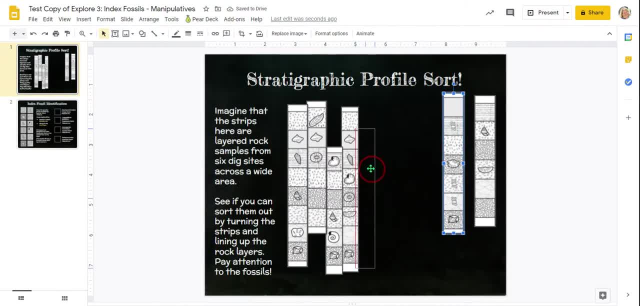 so that that lines up better with that layer, and then, and so on and so on. so you're going to do that with all of these: try to get them where they belong. um, there you go. so that's what mine look like. so now you've got them all lined up, now you can go ahead and go on to the second one. 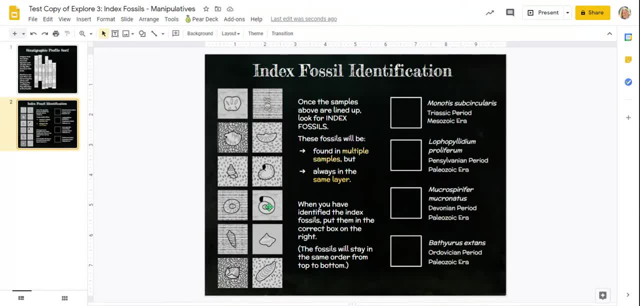 so when you go to the second, you see a lot of the same fossils are now shown here on the site, and these are the things that you can move on this slide. okay, nothing else can be clicked on. you'll notice you can't move anything else. so what you want to do is you want to go back up. 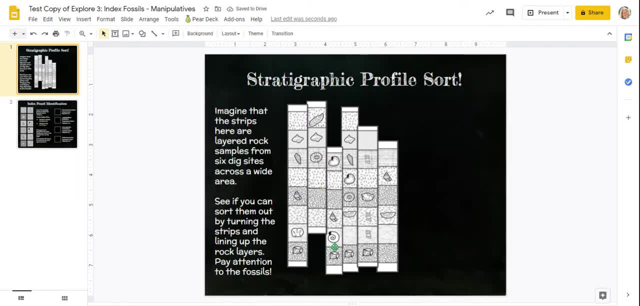 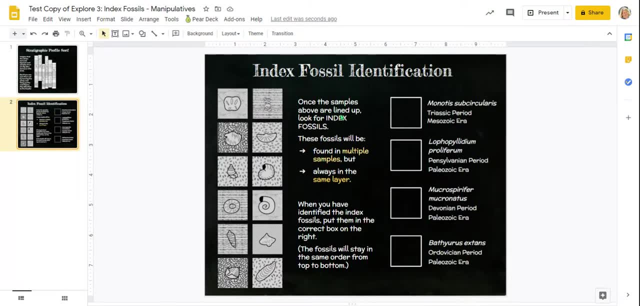 and you want to find which fossils of all the fossils shown here are what would qualify as index fossils. so in order to figure that out, you need to read your instructions here. this is once they're lined up. look for index fossils. they are fossils that will be found in multiple 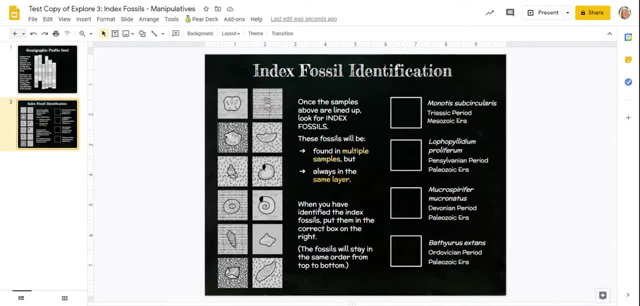 samples. that means you can find them in more than one of those vertical strips, but they are always in the same layer. okay, so if it's in the the squiggly layer, you never find it in the stripey layer, and if it's in the flecked layer, you never find it in the like gray layer. so when you go up, 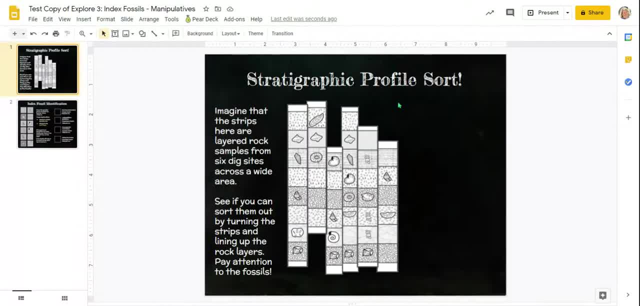 here. i mean it's best to start at the top and work your way down because, again, whatever's near the top is the youngest, whatever's near the bottom is the oldest, and it's best to work from top to bottom. so, um, we have this fossil here, but that's just one lonely fossil by itself, so that's not in. 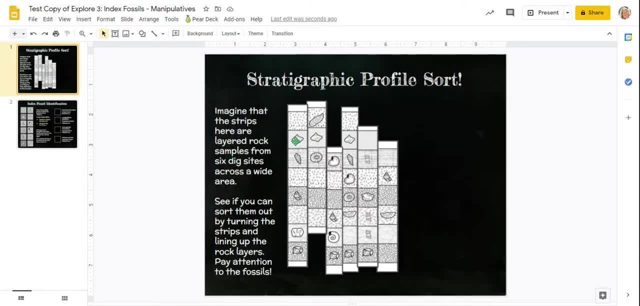 multiple strips. you cannot use that as an index fossil. but the next fossil we run into is this kind of swervy sea creature. i'm not sure what that is- um on the gray background and notice that there are three of them: this strip, this strip and this strip all have it. but you don't see that. 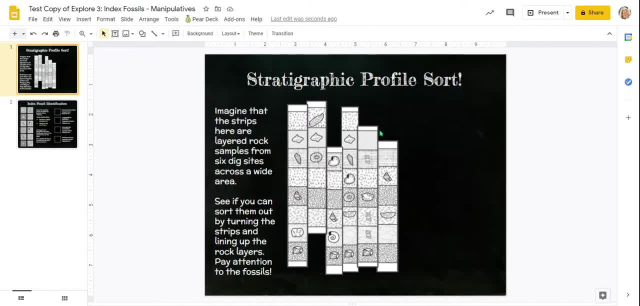 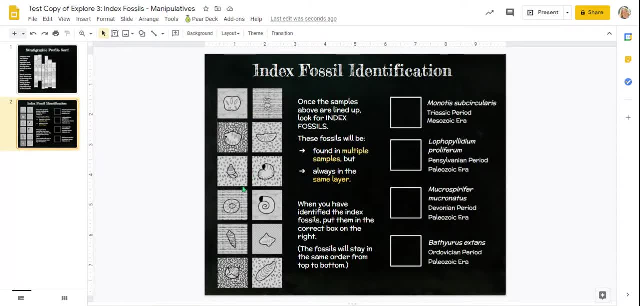 fossil on any of the other layers down here. so that means that is definitely an index fossil. so you want to kind of take note of what that looks like. and then you're going to go to your second page, find that fossil in the list and here it is and you're going to move that into the top. 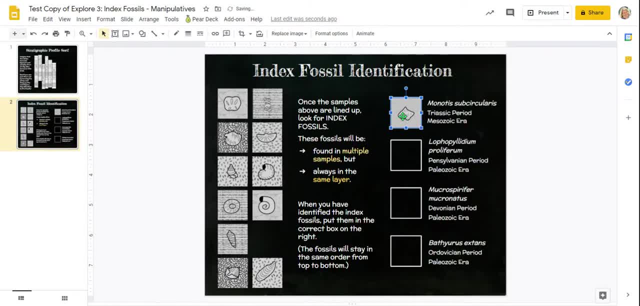 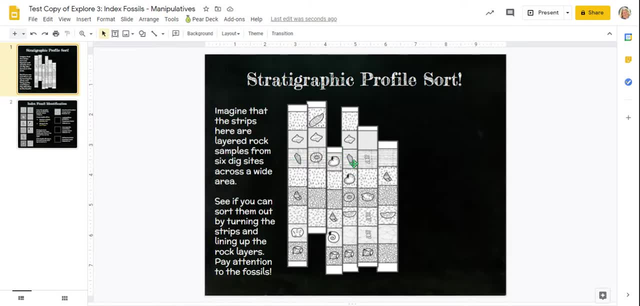 box, because that was in the top most layer, that where we found any. okay, so that's number one. and then you're going to do that again, you're going to come back here and you're going to look down to the next layer like, okay, so now i see there's this kind of corkscrew thing, but there's.